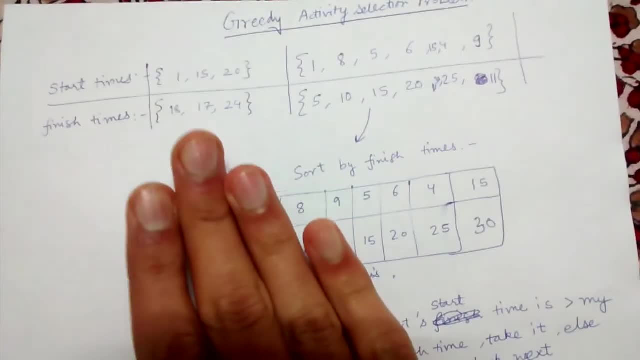 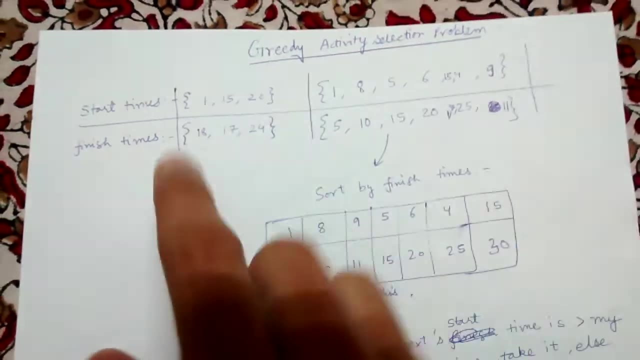 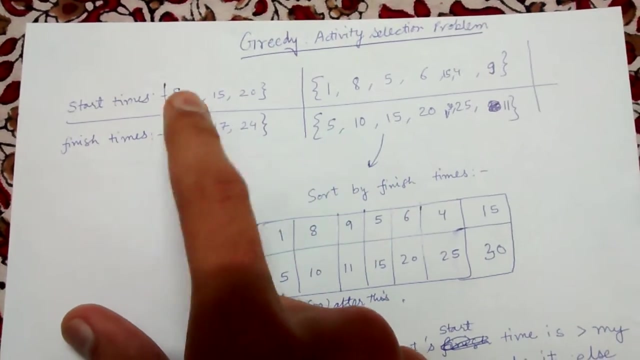 present choice and choose whichever the best choice is. So what activity selection problem is? let me describe So in this. you are given a few activities. In this case we are given three activities and their start and end times are given. So let's say this is an activity. 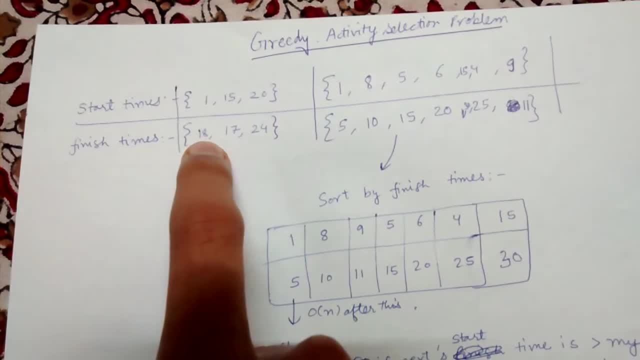 which start time is 1 and end time is 18.. So let's say this activity is 1 and end time is 18.. So let's say this activity is 1 and end time is 18.. So let's say this activity. 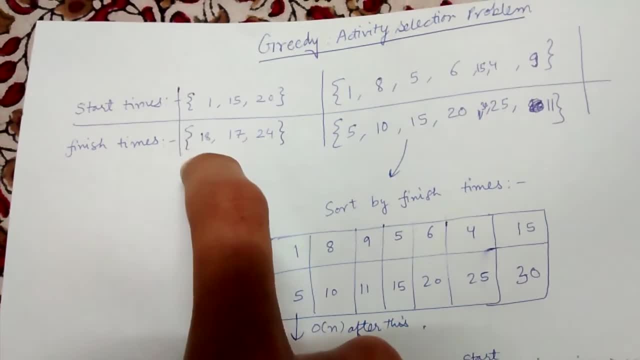 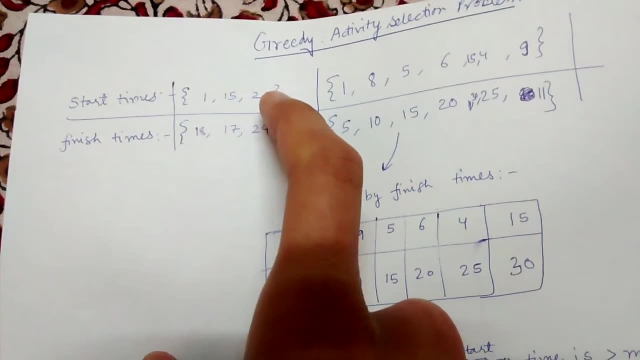 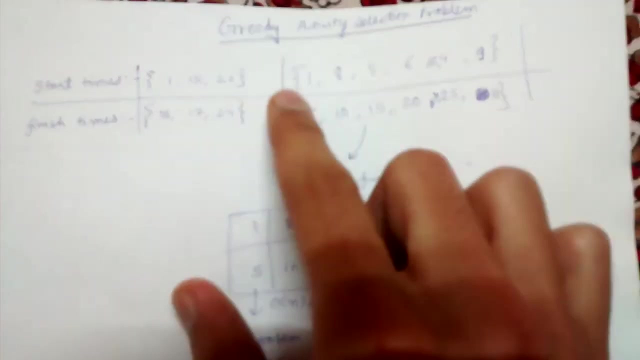 is breakfast, which starts at 1 and ends at time 18.. This is lunch, which starts at 15 and ends at 17.. And dinner, which starts at 20 and ends at time 24.. Similarly, here we are given seven activities and their starting and ending times are given. So these are all. 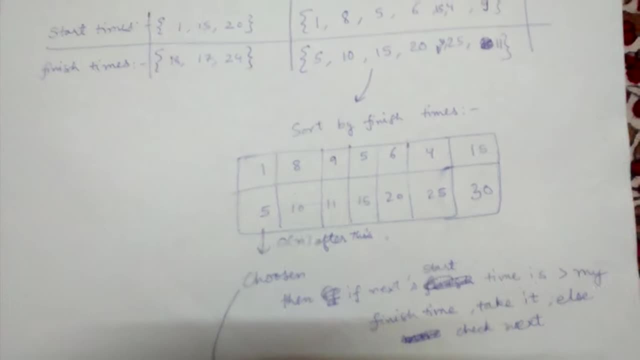 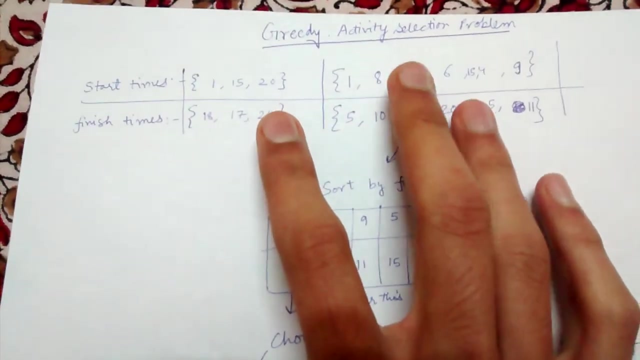 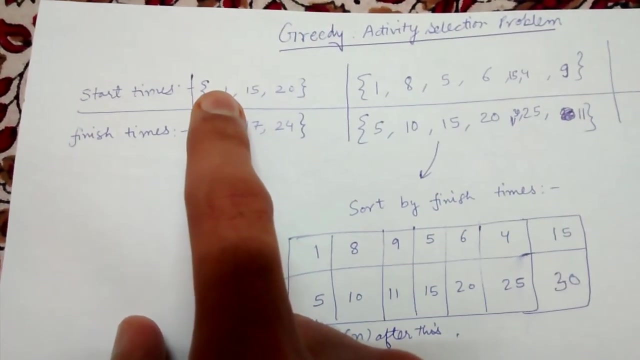 pairs, as you can guess. So how to solve? so now, our aim in this group is to find all the activity selection problems. So here, the activity selection problem is 1: I am a person and I want to do maximum number of activities so that no two of them overlap. 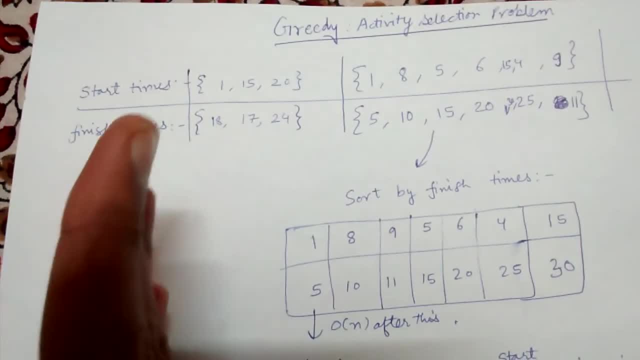 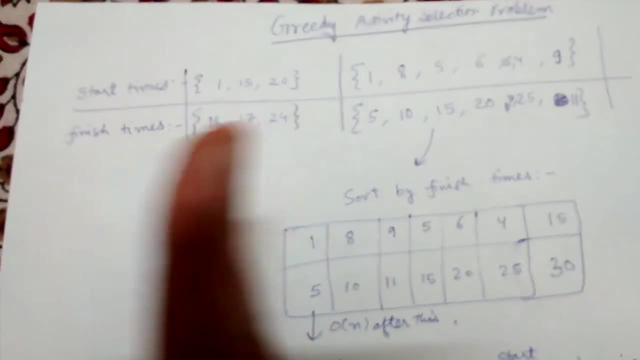 So let's say I have done 1 to 18.. Then I am occupied from the time 1 till the time 18.. I can't do anything between that time. So 15 to 17 is the time which is overlapping with 1 to 18.. It lies between 18 and 18.. This is the time which is overlapping, with 1 to 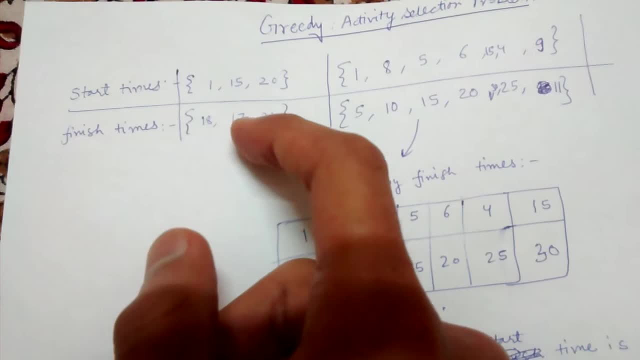 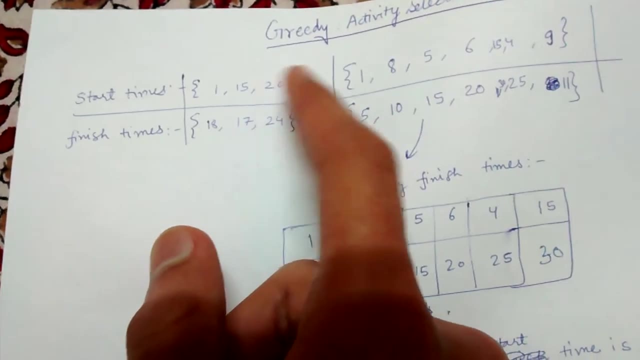 18.. So with that you can find out that the number of activities is the same as the number of that interval. so I can't do this activity now if I choose to do 1 to 18, but I can still do 20 to 24, because 20 to 24 is completely out of this 1 to 18. 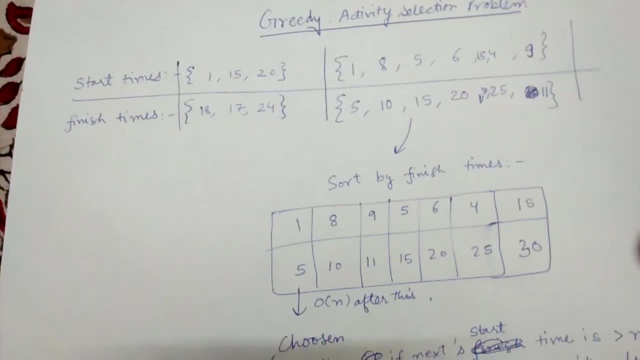 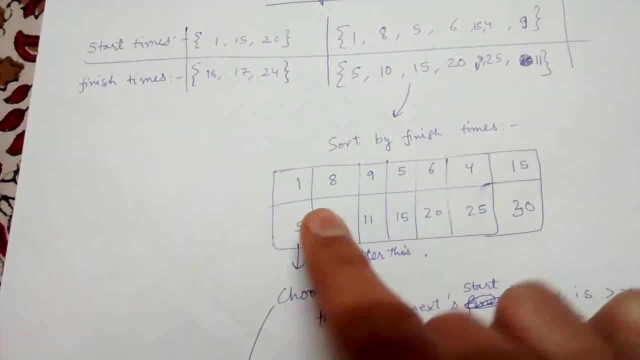 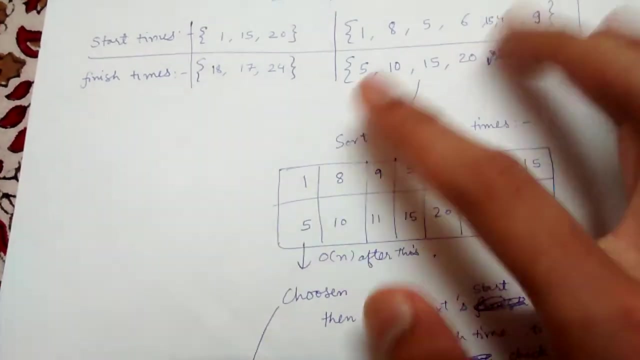 range. okay, so how to solve this problem? we sort the activities by their finish time, so these pairs are sorted by this finish time. so 1 to 5, this is having the lowest finish time. so 1 to 5 come here, then 8 to 10, next then come this, 11, this 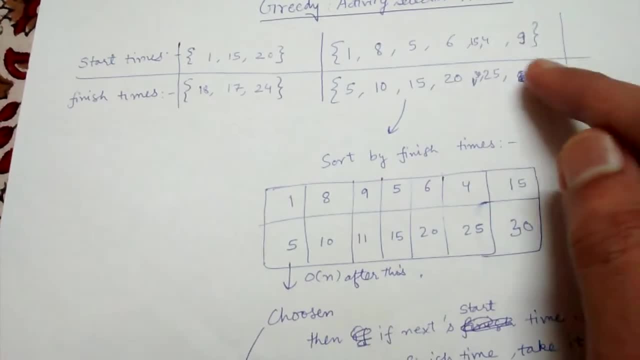 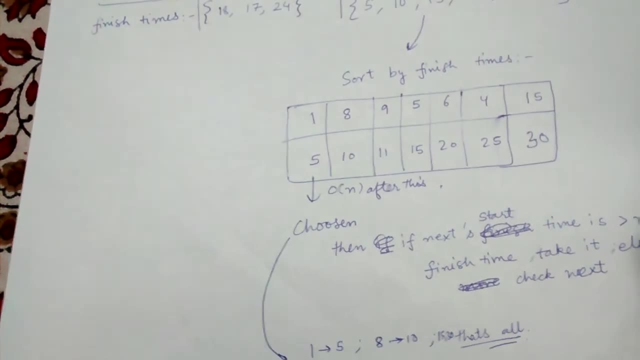 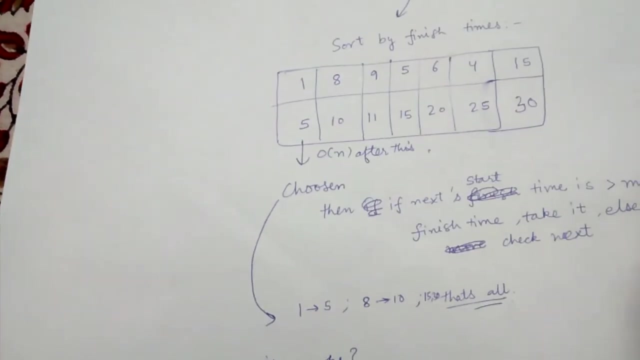 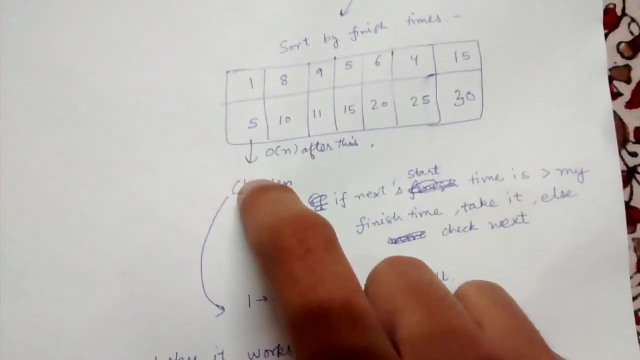 is having the next finish time. so 9 comma 9 to 11, this activity comes here, and so on. so sorting will take o and log n. if you use a optimal search algorithm like merge sort after this one time will be required. so what we do is we really choose the first one, the first activity. we 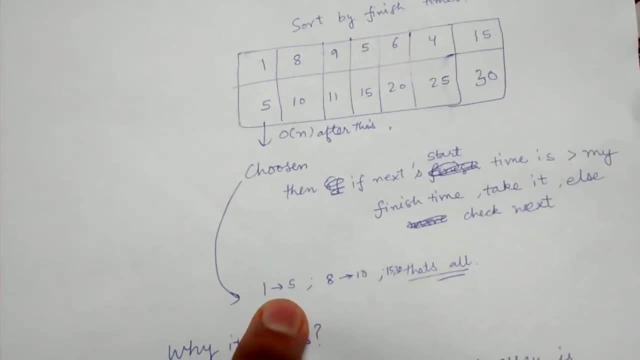 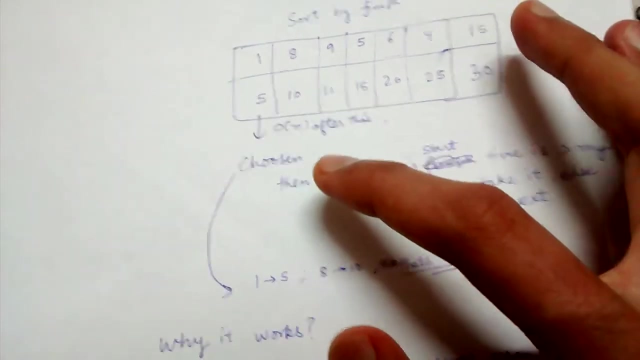 trivially choose it. so first activity is chosen, 1 to 5 is chosen. then, if next start time is greater than my finish time, so I am the current and the next activities start time is greater than my finish time. my finish time is 5. next. 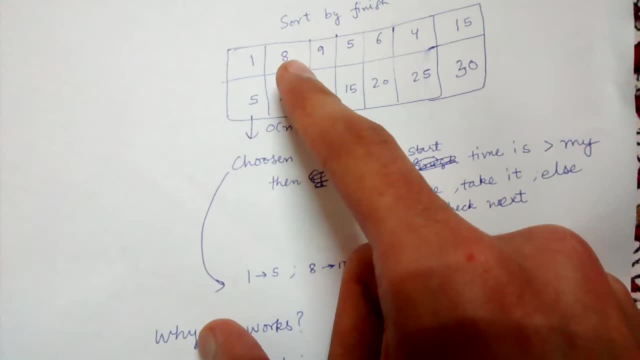 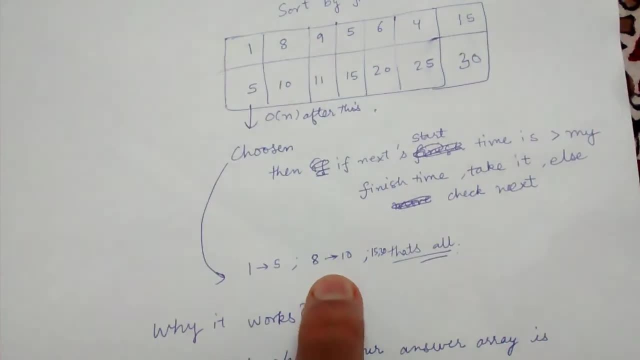 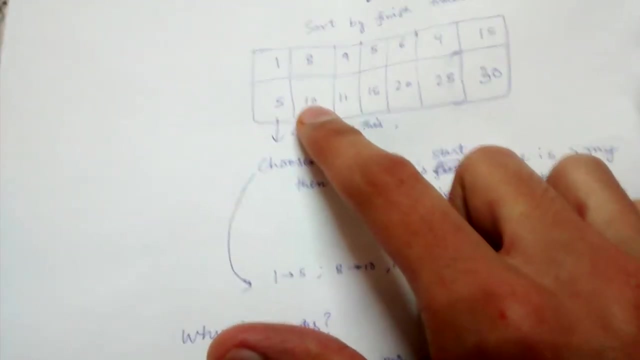 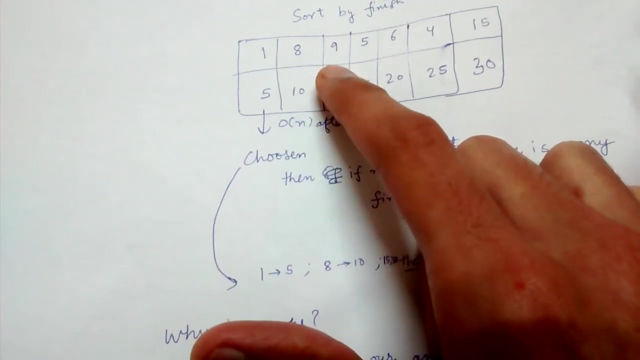 start time is 8, which is greater than 5, so I can easily do this also, so I I choose it 8 to 10. now 8 to 10 becomes my current activity. now let's move further. I see 9 to 11. my finish time is 10, but next activity start time is 9, so I will be ending at 10, so I can't pick up. 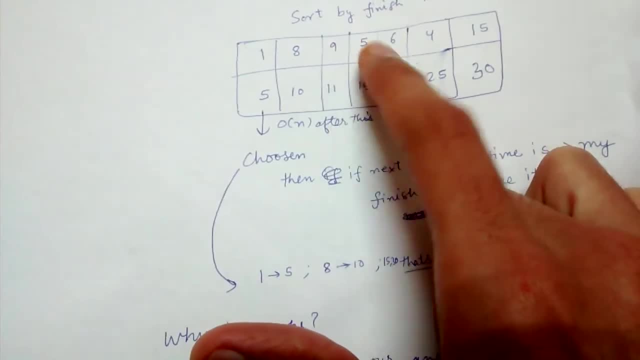 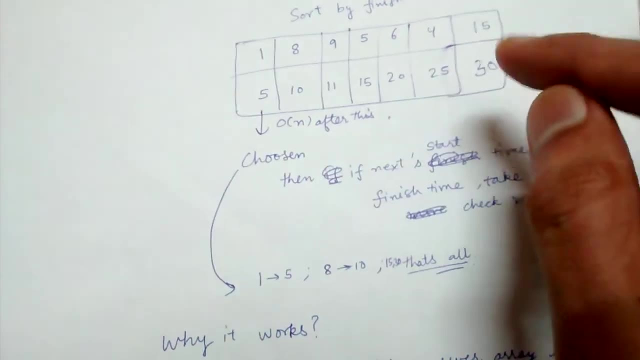 an activity which starts at 9, so I can't take this. so I move further. 5 to 15: this also I can't take, because 10 is greater than 5. 6 to 24: this also I can take, this also I can't take. so I come. 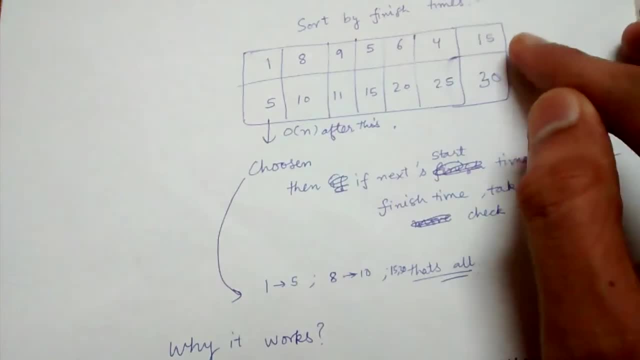 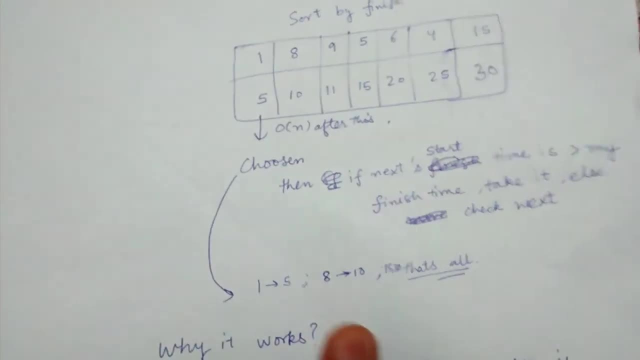 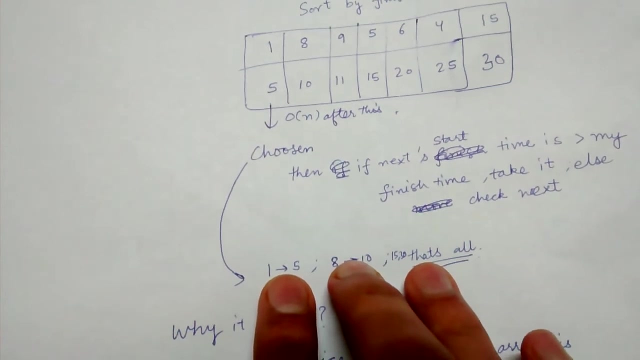 here. 15 is greater than 10, so this activity will be started after my 8 to 10 activities finished, so I can easily pick up this activity. so 15 to 30 is the next one, that's all. so I can pick up maximum of three activities in this case. this is the optimum solution and this is the answer. 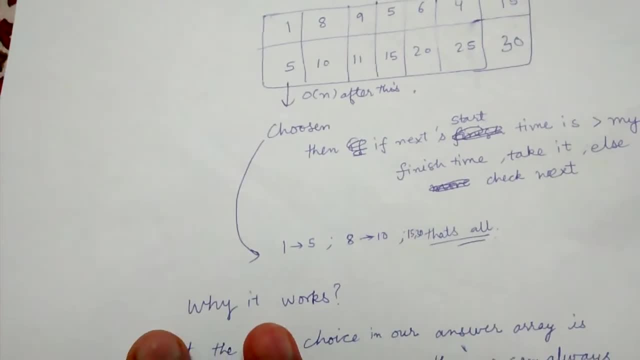 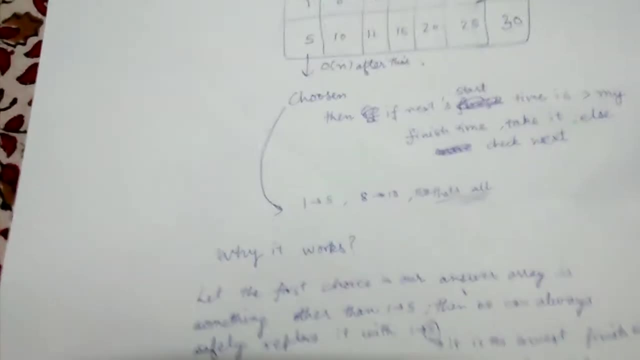 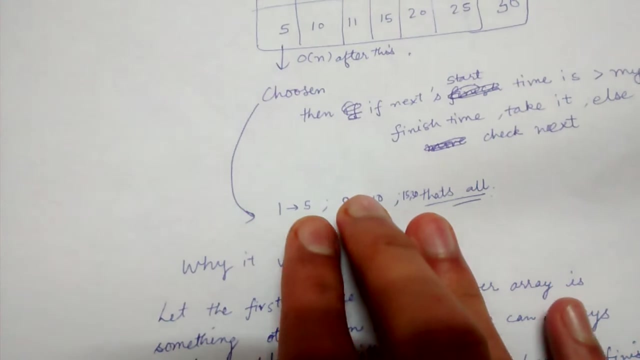 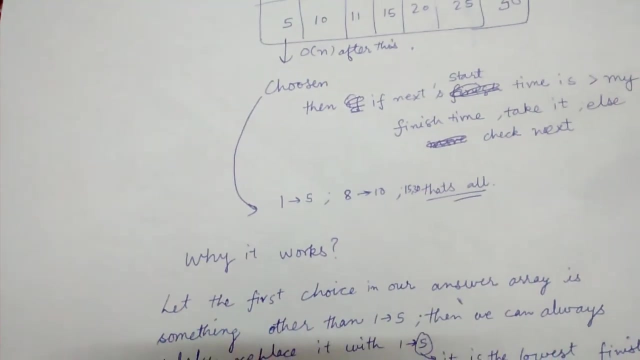 actually so why it works, choosing the first one and then greedily choosing whatever comes the first, because let the first choice so our answer, let us assume the first entry in our, so there can be multiple optimum answers in this case. but what we have given, we want to show that this. 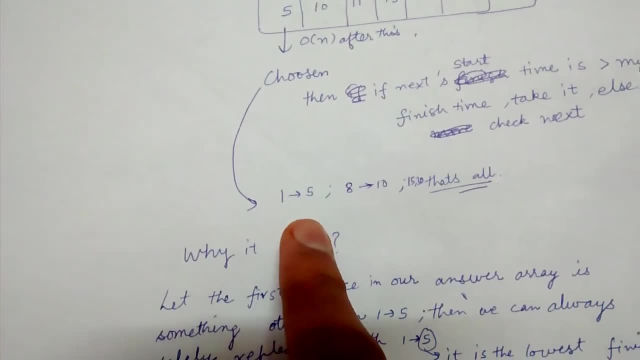 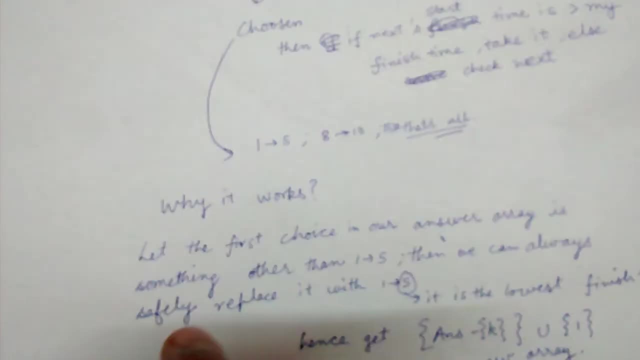 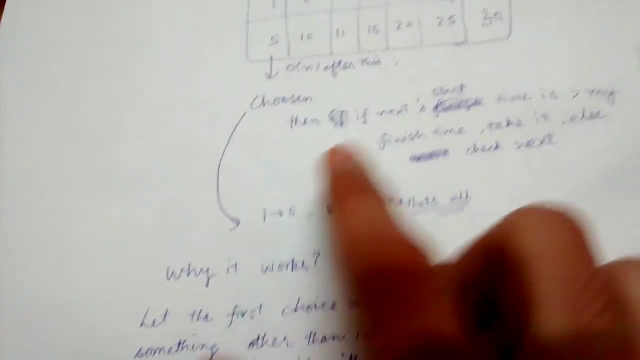 is an optimum answer, so that the first choice in our answer is not 1 to 5, it is something other than 1 to 5, then we can always safely replace it with 1 to 5. key difference is difference in practice, so that you can see why is it so. because if